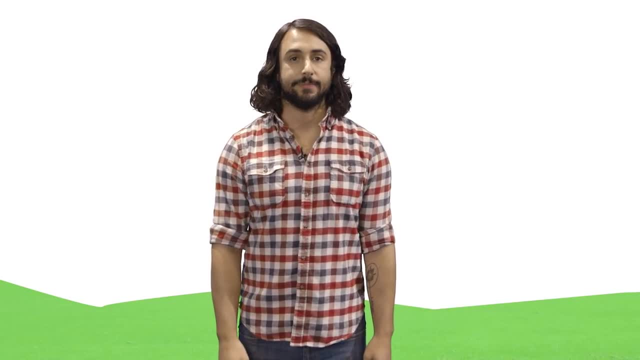 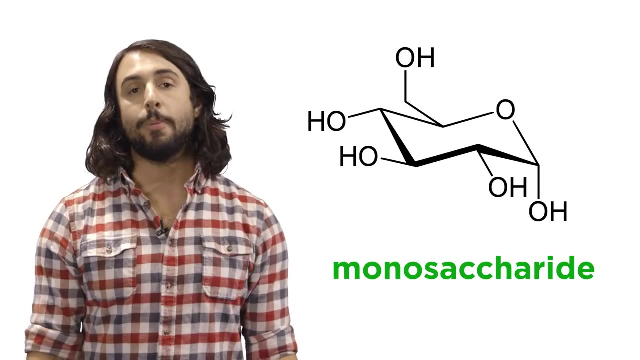 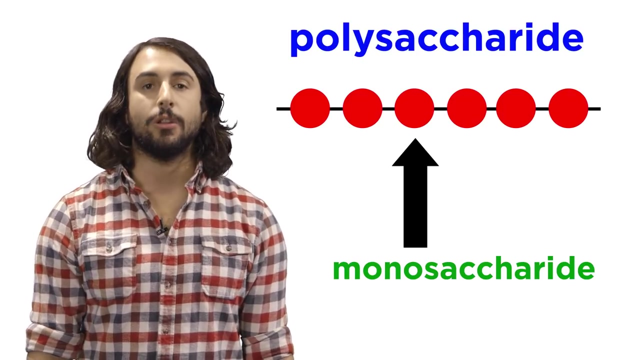 Hey guys, it's professor Dave. let's discuss polysaccharides. Carbohydrates include simple sugars like monosaccharides, but they also include polysaccharides, which are long polymers of these simple sugars, So we need to understand the way they polymerize. 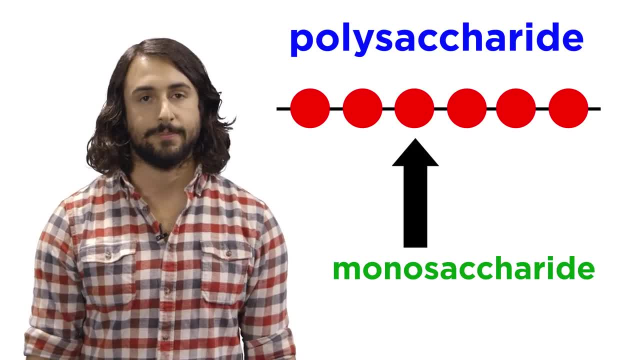 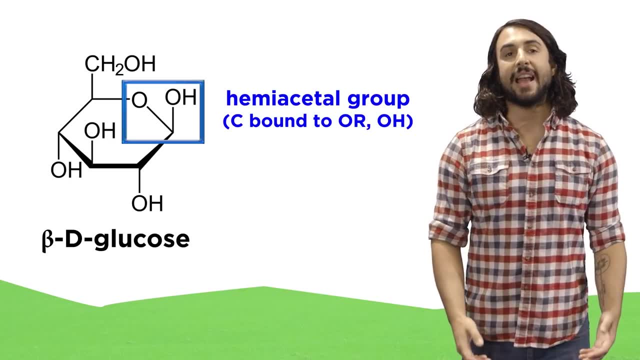 as well as certain characteristics of the resulting polymers. First let's return to our Hayworth projection for beta-glucose. In the cyclic form we can see there is a hemiacetal group, and if we remember the mechanism by which a hemiacetal will become an acetal. 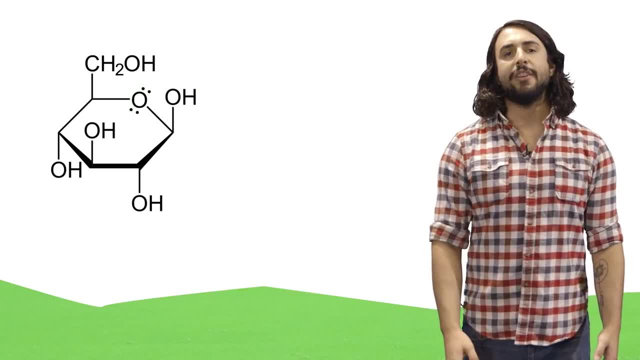 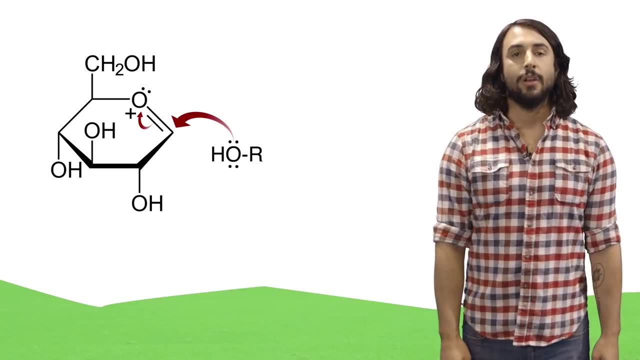 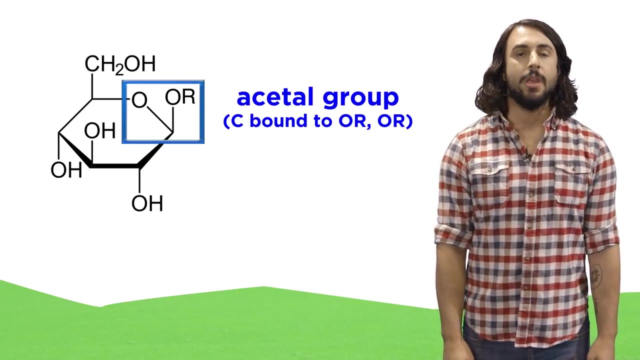 that is essentially what will happen here. We know that if this hydroxyl is protonated, it could leave, and then this carbon could be attacked by an alcohol, forming what we call a glycosidic bond as well as an acetal functional group in the process. 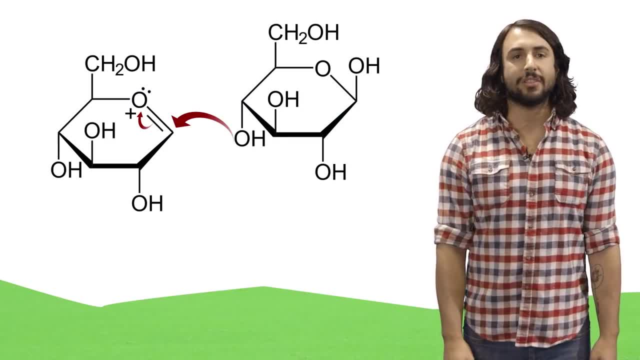 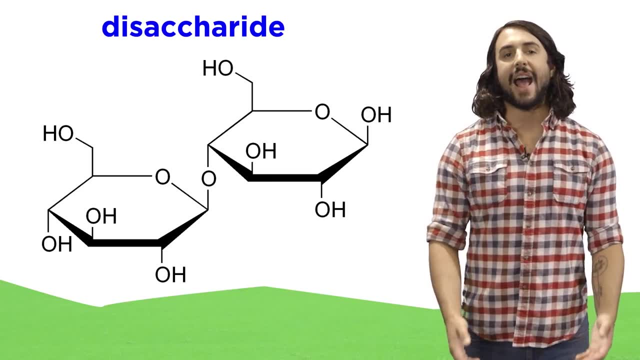 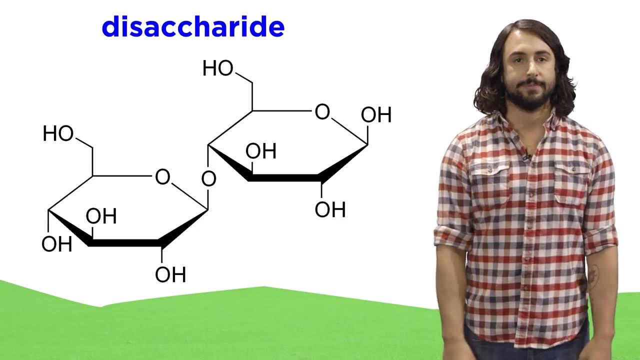 But if the alcohol that attacks is one of the hydroxyl groups, on another monosaccharide we will get a disaccharide. This is still an acetal functional group, but it links two monosaccharides together via a glycosidic bond. Here we have a beta-glucose linked with. 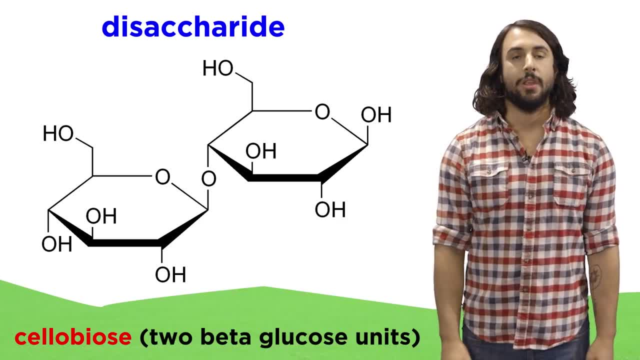 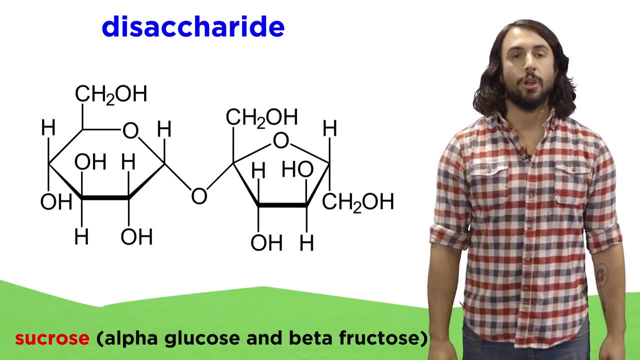 another beta-glucose, which makes cellobios. Other common disaccharides are lactose, which is beta-galactose and alpha-glucose, And sucrose or table sugar, which is alpha-glucose and beta-fructose. 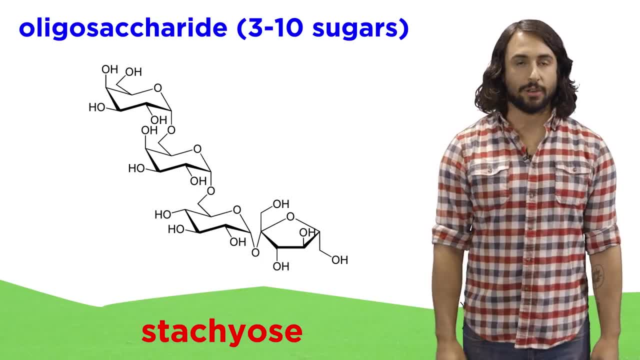 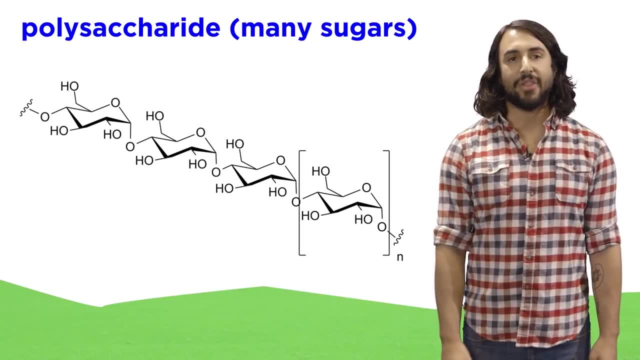 We could continue to polymerize further, making an oligosaccharide which will have three to ten saccharide units, or a polysaccharide. Polysaccharides can have thousands of monomeric units, and nature uses these quite frequently. 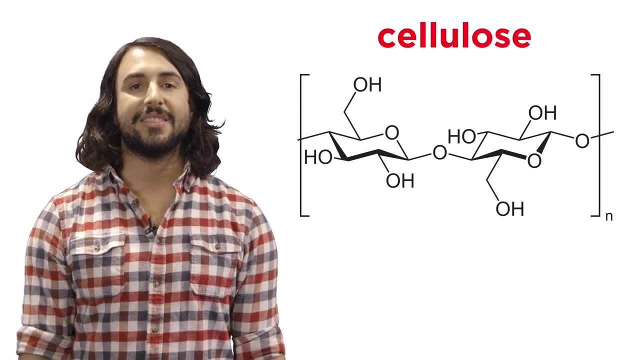 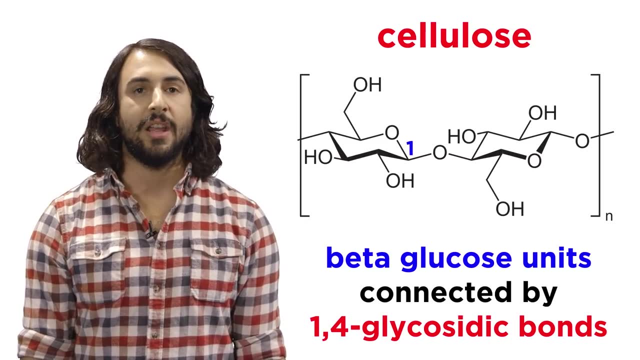 For example, cellulose, which is abundant in plants, consists entirely of beta-glucose units connected via 1,4-glycoside. This means that carbon 1, the anomeric carbon of one sugar, is connected to the hydroxyl.